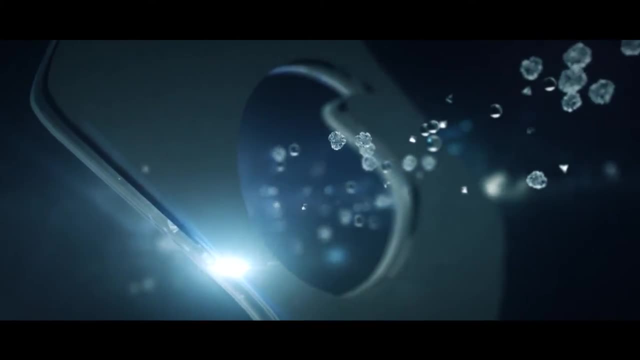 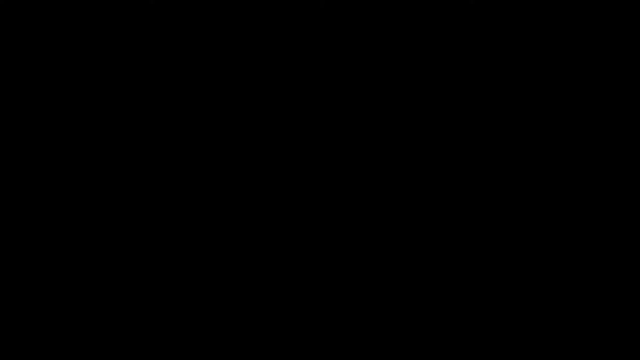 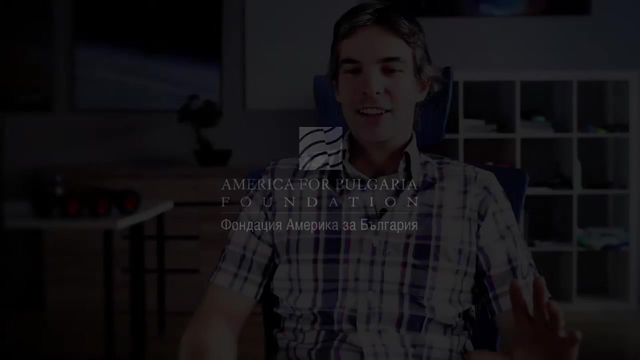 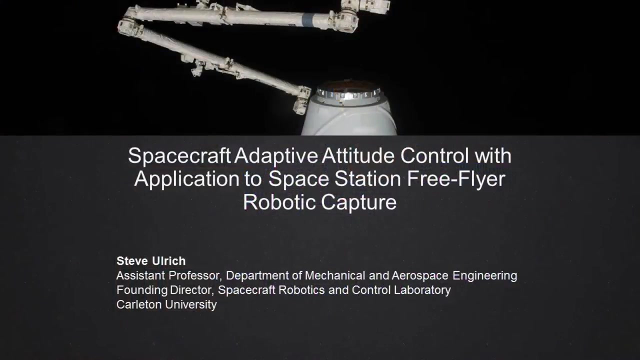 Okay, so this time I'll present a much more detailed application example specifically for spacecraft adaptive attitude control in an actual application to space station free flyer robotic capture maneuver. 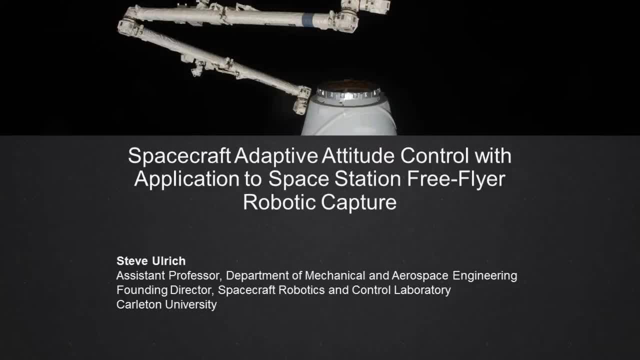 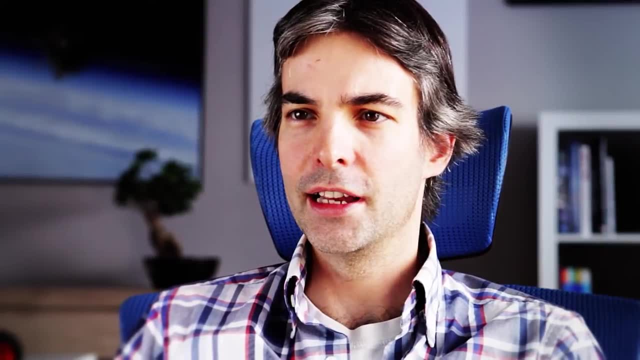 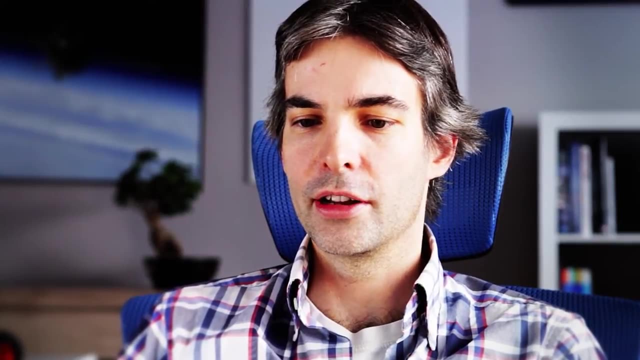 So that's a work that my Ph.D. student and I, so John Feng Shi, my Ph.D. student, and I did with MDA Space Mission in Brampton, Ontario. So MDA is a company that design and build Canadarm 1 and 2. So that's a work we did in collaboration with their GNC department. 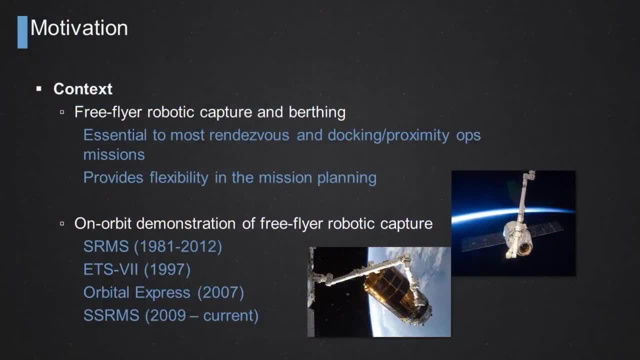 So the context is that, as you may know, using a robotic arm to capture a free flyer vehicle in space is a critical enabling technology that is mostly used for proximity operation and rendezvous mission scenarios as well. And the key thing is that it provides some flexibility in terms of the mission planning. And I'm sure you're aware as well that previously there has been some on-orbit demonstration of free flyer robotic capture maneuvers in space starting from SRMS, so Space Shuttle Remote Manipulator System, or Canadarm 1, starting in the early 80s up to three years ago, 2012. 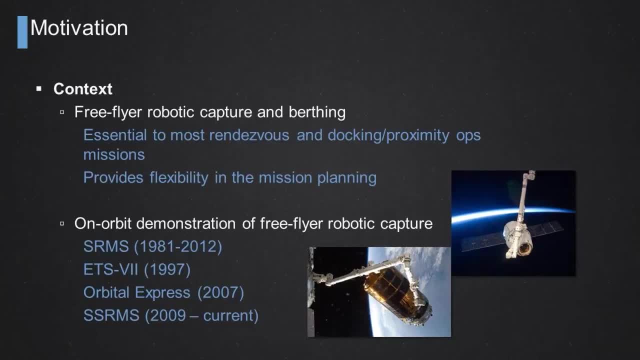 There was another experiment in space called the Engineering Test Satellite 7 back in 1997 by the Japanese Space Agency, JAXA. More recently with Orbital Express, that was a DARPA and Boeing experimental mission that looked at robotic technologies in space, among other things how to robotically capture a satellite. 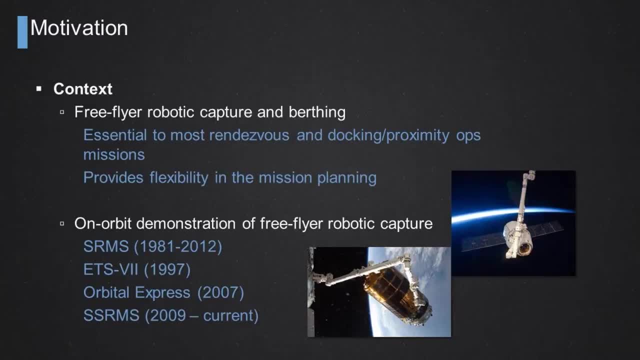 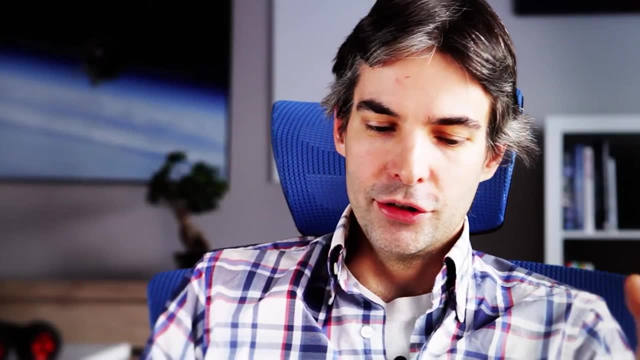 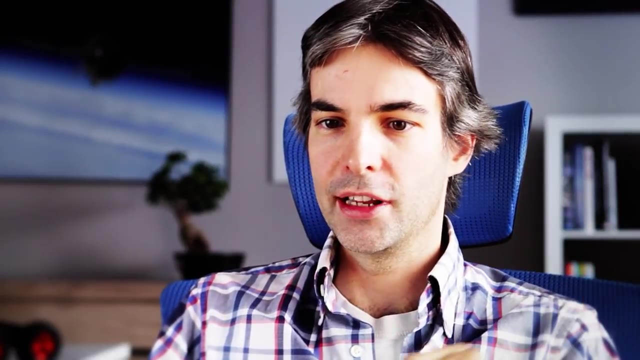 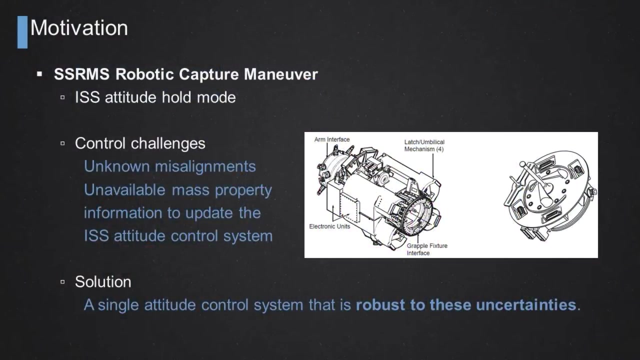 And also more recently with Canadarm 2, or Space Station Remote Manipulator System, SSRMS, from 2009 up to now. But when you're trying to capture a free flyer vehicle with a robotic arm in space, the way at least it works for the ISS is that the space station is placed into an attitude hold mode, implying that there is an attitude control system onboard the ISS that uses the ISS control moment gyroscopes that I've talked about earlier to regulate its attitude as much as possible regardless of the robotic maneuvers that are taking place. 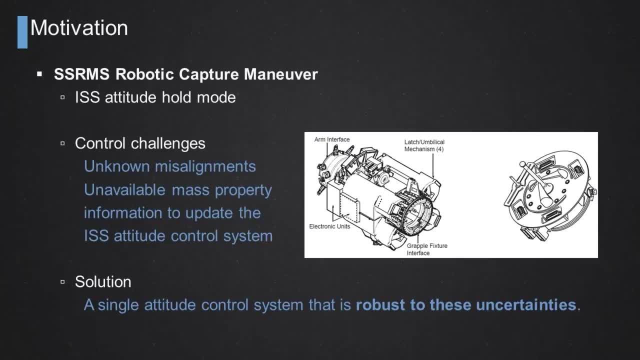 And from a control perspective, there are many challenges inherent. 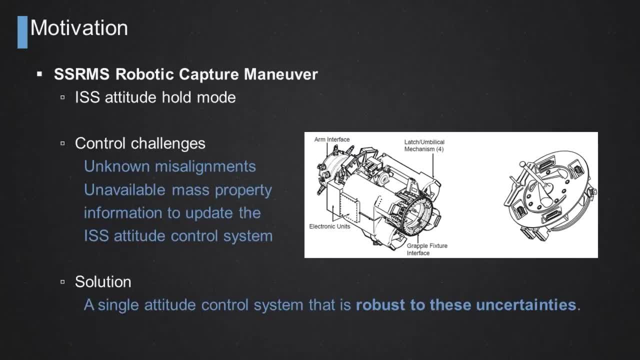 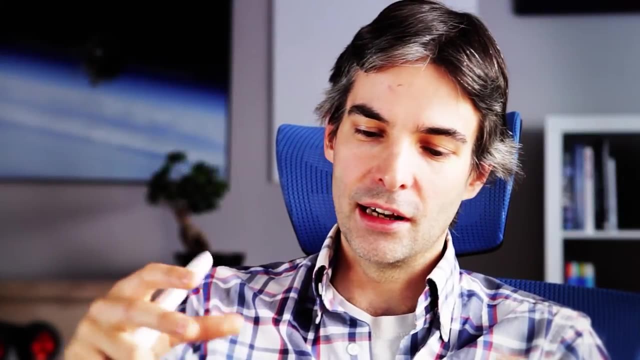 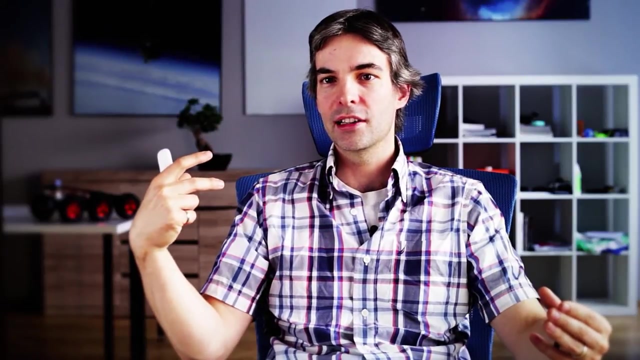 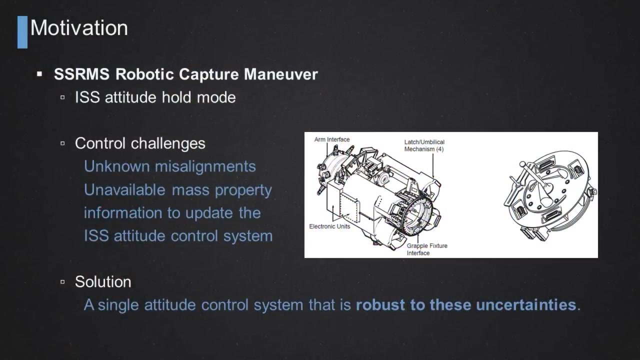 To a robotic free flyer capture maneuver. In that case, there might be some misalignments between the latching anti-factor at the end of the robotic arm and the grapple fixture installed on the target free flyer vehicle. So the greater the misalignment between those two interfaces, the greater the external perturbations as seen on the robotic side, so as seen from the chaser perspective, will be. Also, if you're trying to capture with a robotic arm a free flyer vehicle, you may not know exactly its mass properties. And if you have one robotic arm trying to capture different vehicles, well, they will all have their specific mass properties. 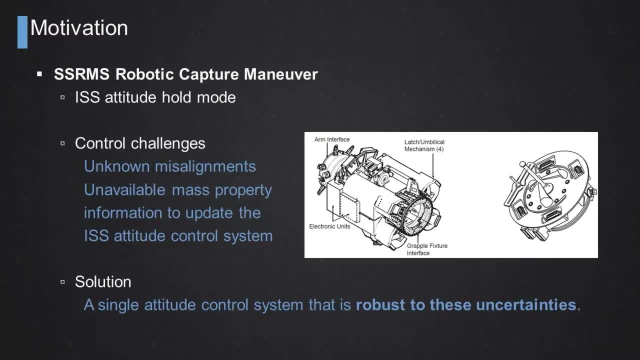 So the idea is that you may not be interested in redesigning your attitude control system that will ensure that the attitude of the robotic platform is as stable as possible. 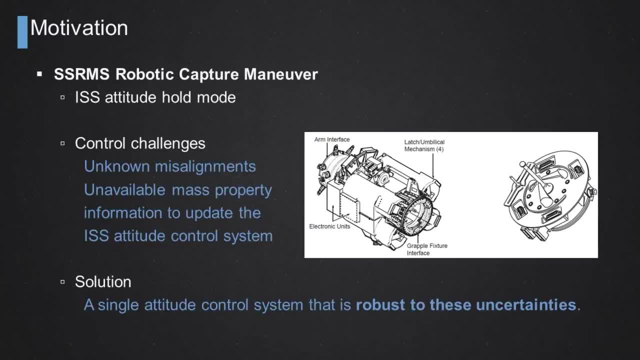 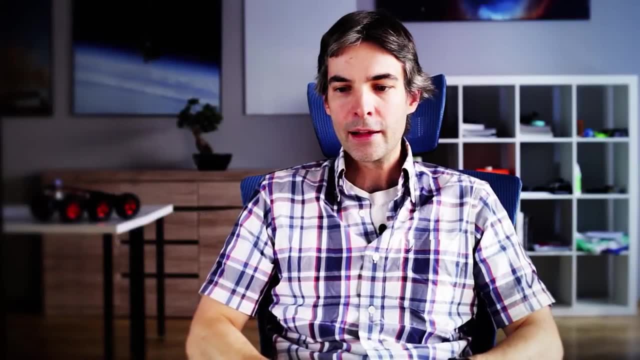 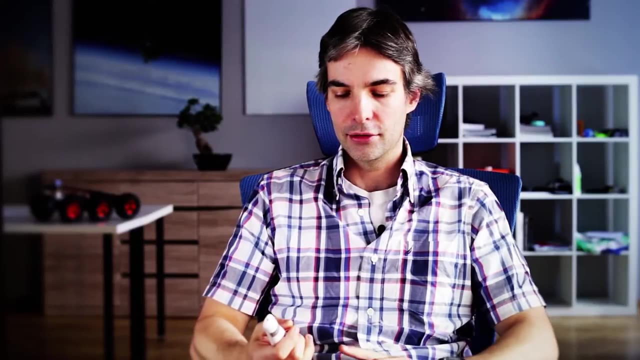 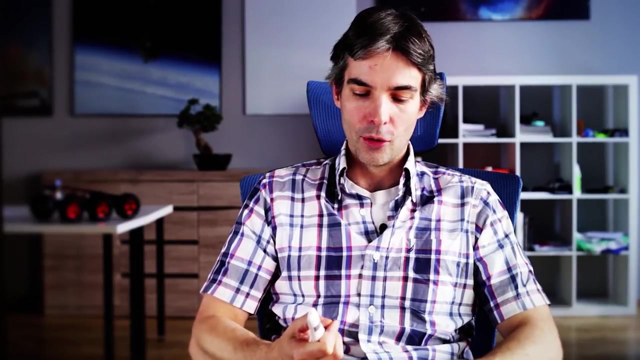 So you do want to use a single attitude controller regardless of the fact that the robotic arm might be trying to capture different free flyer vehicles. So in other words, you want an attitude control system that will be robust to that kind of uncertainties. So robust to the fact that you may not know the mass properties of the target vehicle you're trying to capture. And robust to the unknown misalignments between the latching anti-factor and the grapple fixture. 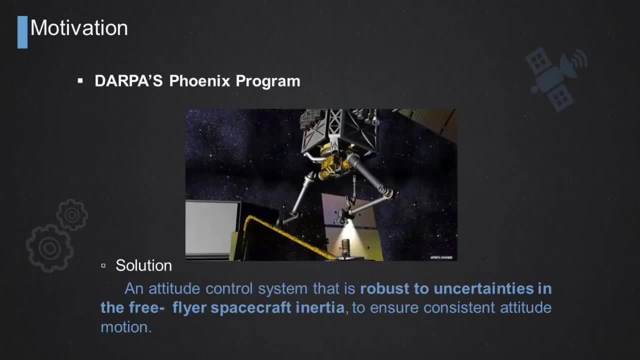 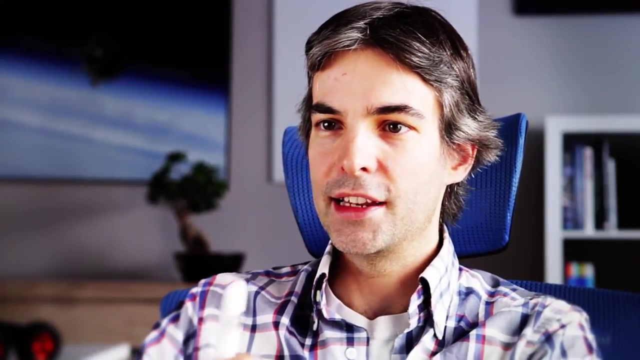 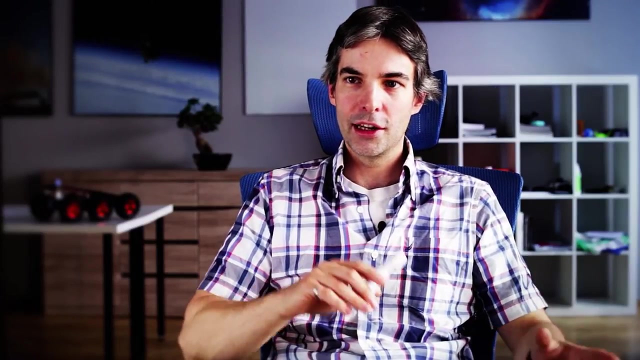 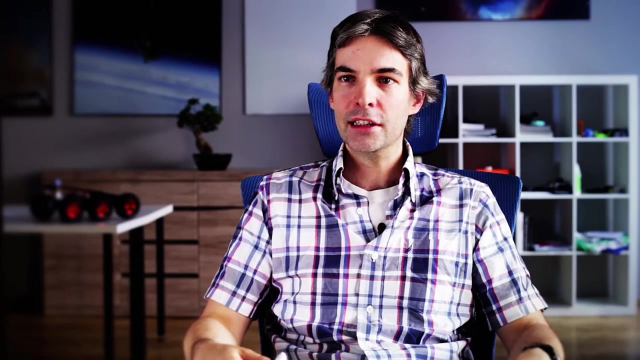 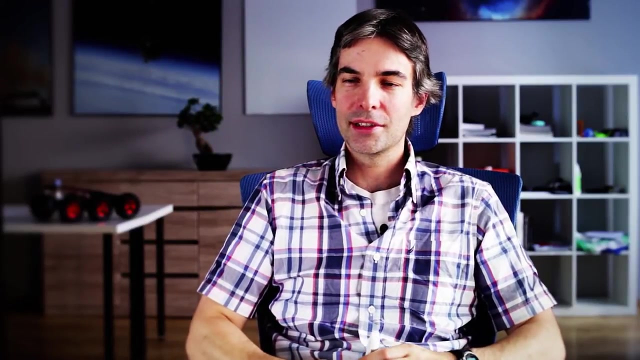 So another example of such robotic capture maneuver is related to the DARPA's PHOENIX program. And the objective of this program is to have what's called a satellite. So that's a miniature satellite equipped with a robotic arm that will go and capture some parts of a depleted large geostationary satellite to then assemble a new satellite or a new aperture based on the different components those satellites will detach from the target vehicle. And in that case you do want your attitude control system that controls the orientation of the robotic servicer vehicle to be robust to the uncertainty in the mass properties of the chaser satellite because as it's picking up components here and there of the geostationary satellite its own mass and its own inertia properties will change with time. 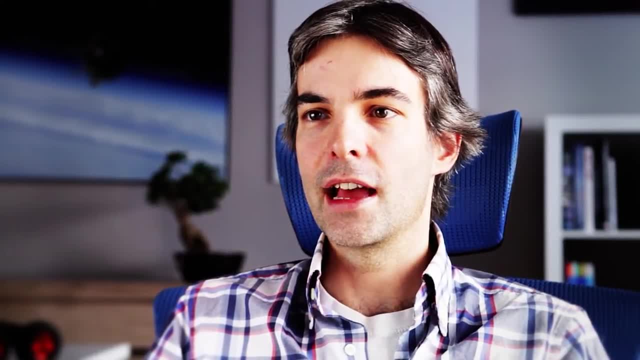 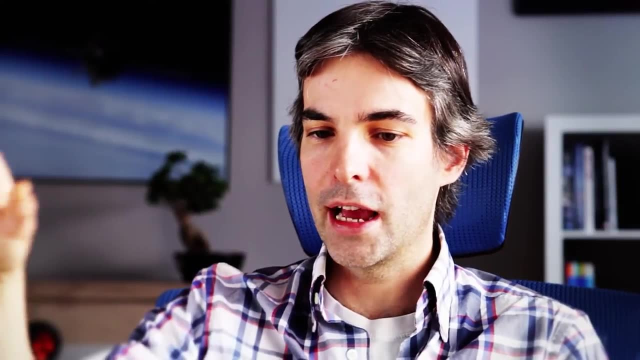 So we do want to ensure that you have a consistent attitude motion regardless of these unknown components that the robotic arms installed on the chaser vehicle will capture. 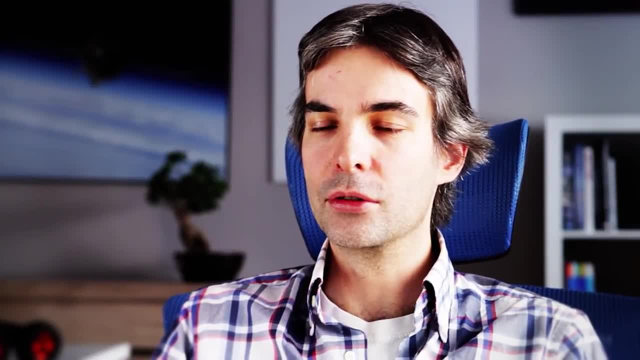 So that's why again we're really looking at having an attitude control system that is robust to those kinds of uncertainties. 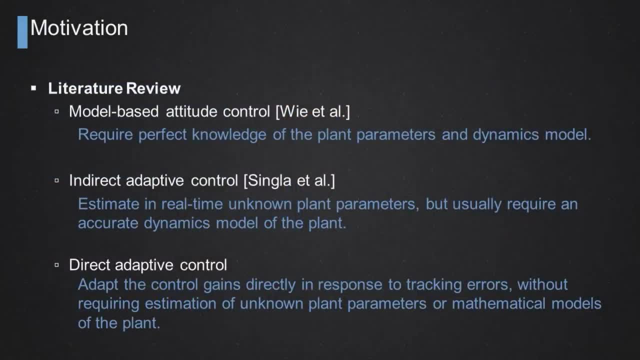 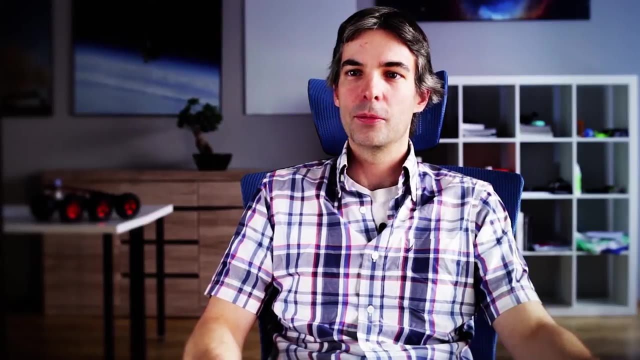 If you look at the literature current attitude control techniques are mostly model based implying that they require perfect knowledge and the planned parameters meaning that the control system needs to know the exact mass properties of the vehicle it's trying to control and needs to know its dynamics model as well. 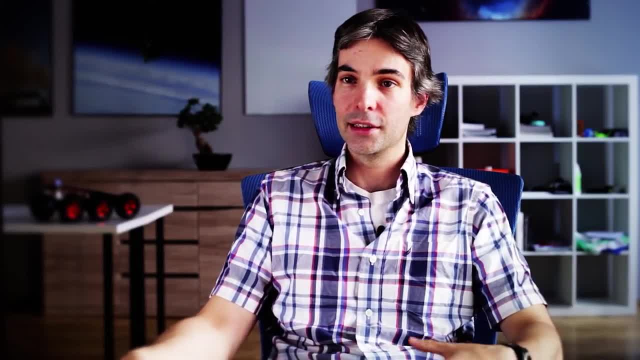 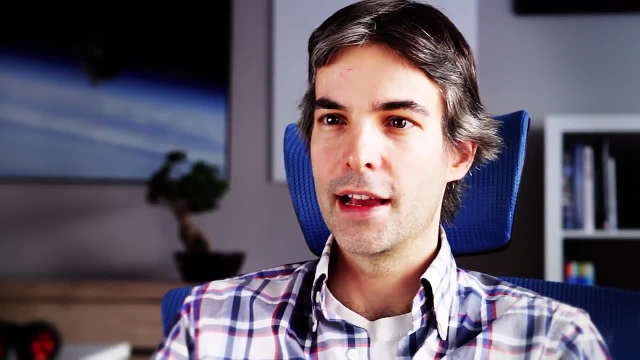 With the result that if you have uncertainties in the parameters say the mass changes or the inertia changes then model based attitude controllers may not work as expected. 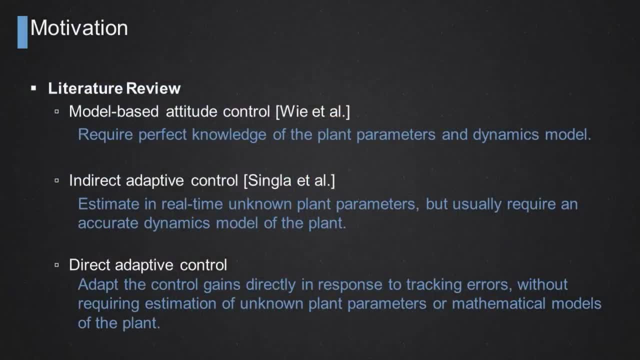 So on the other hand you can cope with these uncertainties by using indirect adaptive control techniques that will estimate in real time the unknown mass and unknown inertia properties of the vehicle the controller is trying to control. 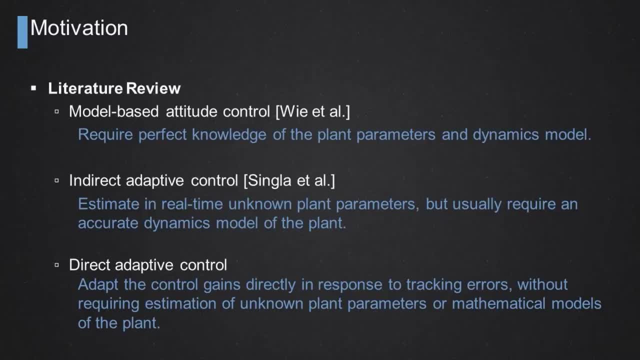 But in doing so you nevertheless need to have access to an accurate dynamics model of the system you're trying to control in that case a spacecraft. 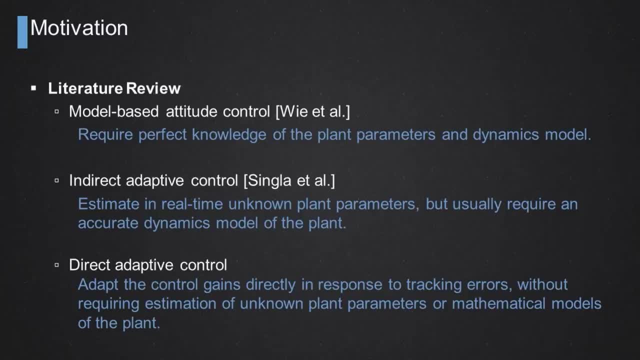 On the other hand you can use direct adaptive control techniques that will adapt in real time the controller gains to make sure that the unknown spacecraft which has an unknown mass and unknown inertia properties due to the fact that it has just pick up or capture another vehicle well the actual response of that spacecraft will match as closely as possible the desired motion as specified by the guidance law. 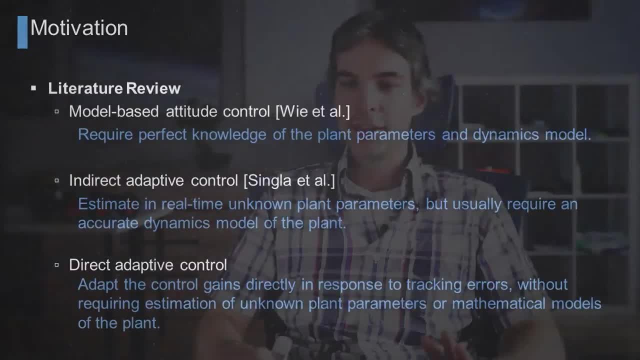 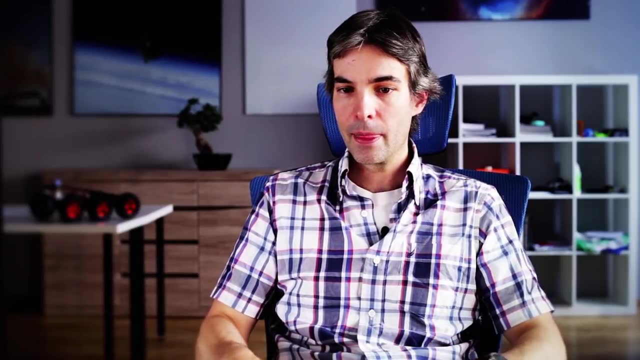 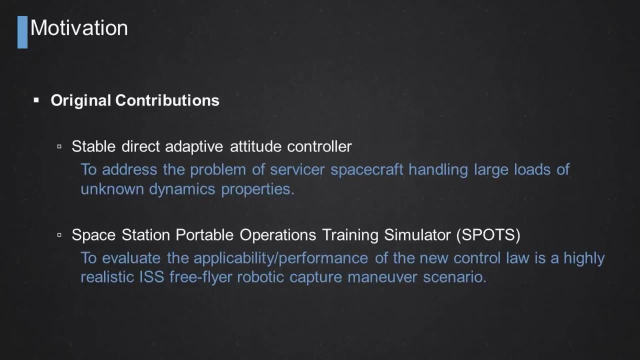 Again regardless of these unknown parameters and regardless of the uncertainty there are certain properties in the dynamics mathematical models of the plant or of the satellite. So in that context the original contribution that we did in the lab here was to come up with a direct adaptive attitude controller that is stable from the theoretical point of view and that also addressed the problem of a servicer spacecraft handling large loads such as another free flyer vehicle that's trying to robotically capture and that has unknown dynamics properties such as mass and inertia. 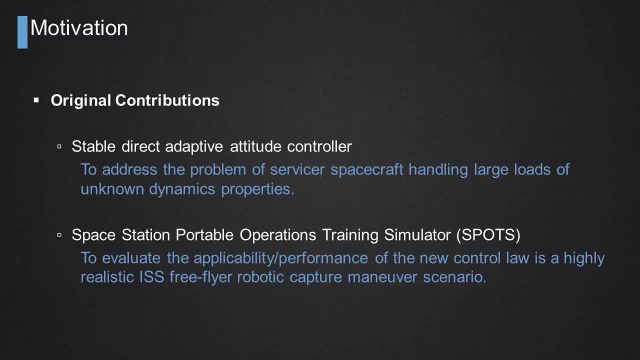 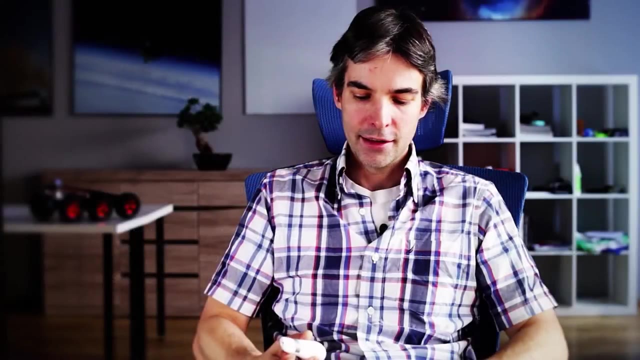 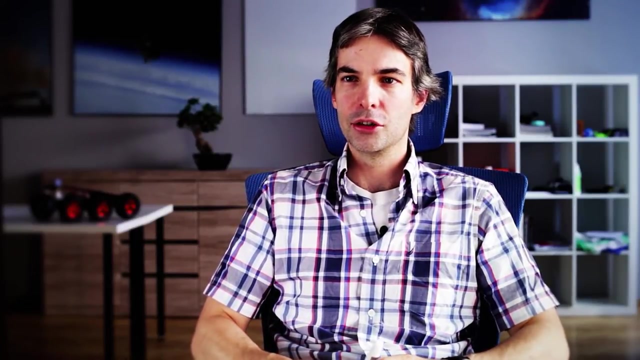 And we also validated our novel approach using the SPOTS simulator. So SPOTS stands for Space Station Portable Operations Training Simulator and that's a facility that's owned by MDA and that's commonly used by the Canadian Space Agency NASA, ESA, JAXA as well to evaluate any robotic maneuvers prior to executing them on a station. 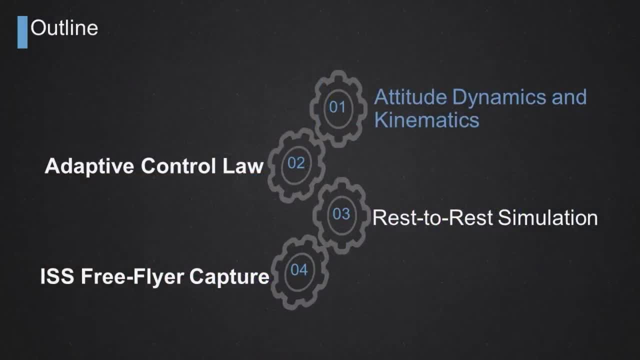 So I broke down this talk into four parts. 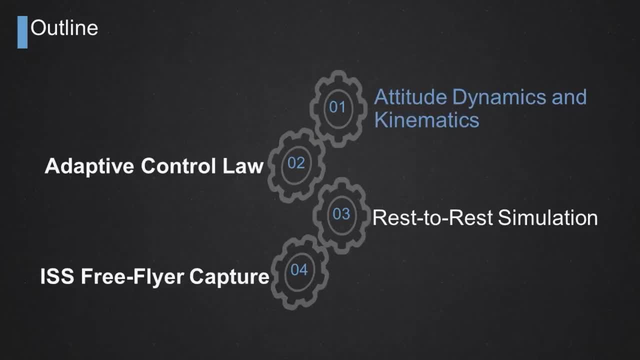 First we'll have a look at the classical attitude dynamics and kinematics equations of motion that predict the attitude motion of a spacecraft. 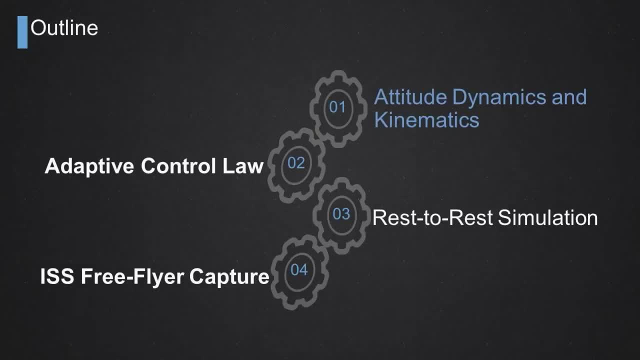 And we'll have a look at the novel adaptive controller that we developed to address a problem of attitude control under off-nominal conditions such as unknown mass properties information and external disturbances. 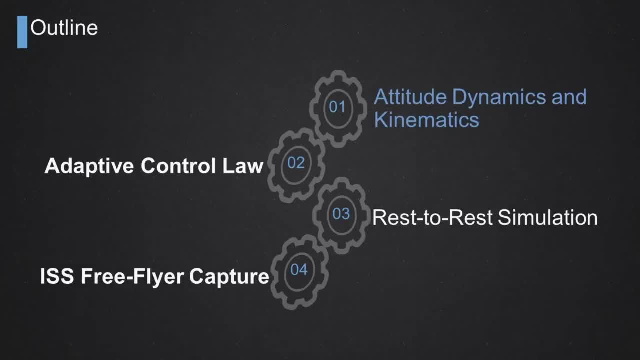 Then we evaluated our novel control on a rest-to-rest simple simulation setup. 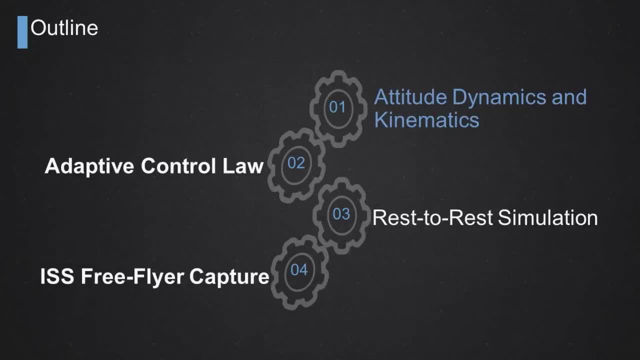 And then we specifically applied it for a space station free flyer capture of the SpaceX Dragon vehicle to see how well our controller was regulating the attitude of the International Space Station during the robotic maneuver. 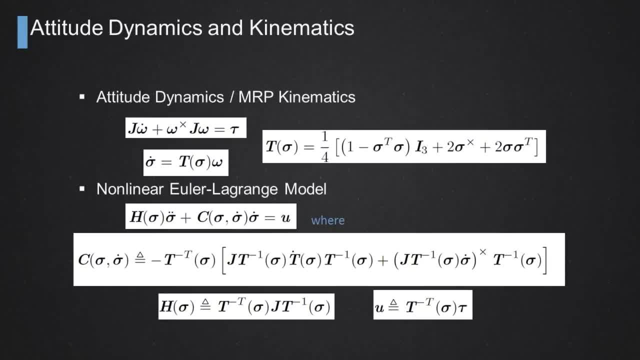 Alright, so that's just a brief overview of the attitude dynamics and kinematics of a spacecraft. So you have J being the inertia of the spacecraft, omega being the angular velocity vector and tau being the control input torque as calculated by the controller. So that's the output of the controller. 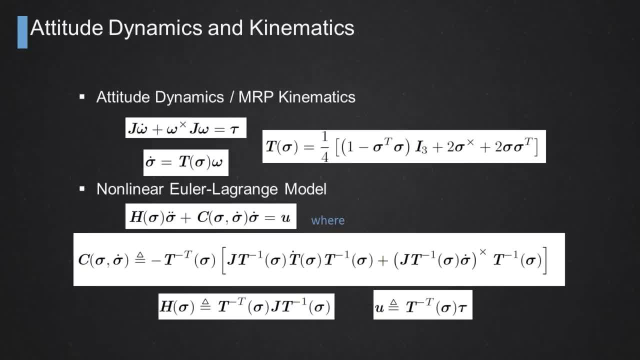 And that's for the dynamics equations. That equation is called the Euler's equation of motion. And in terms of kinematics, so kinematics is just a way to represent the orientation of the spacecraft based on the angular rate vector. So there's no dynamics effect involved. It's just kinematics. 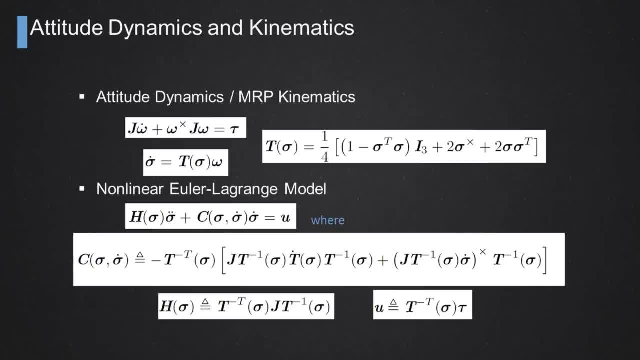 So how to relate the angular velocity vector to the current orientation? 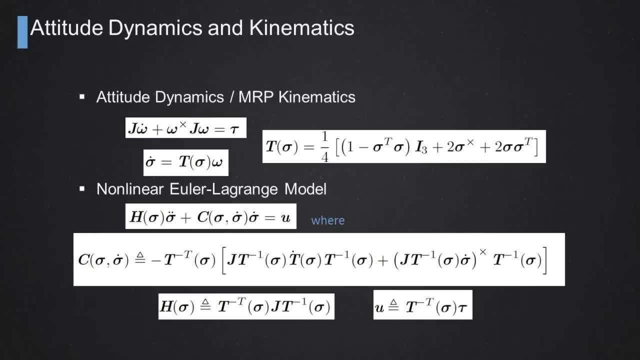 Typically it's done using quaternions. But in this work we opted for using the modified rotor gaze parameter instead. Just because the modified rotor gaze parameters or MRP for short, are a three component vector as opposed to a four component vector for quaternions. 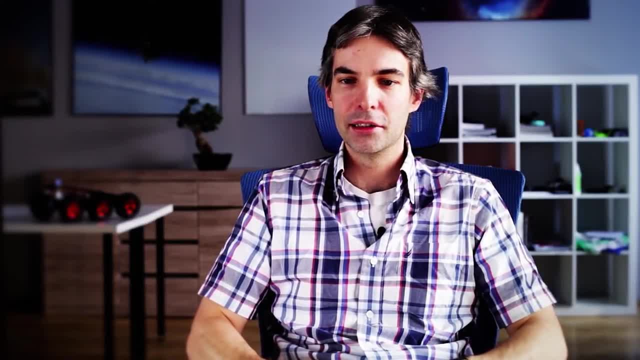 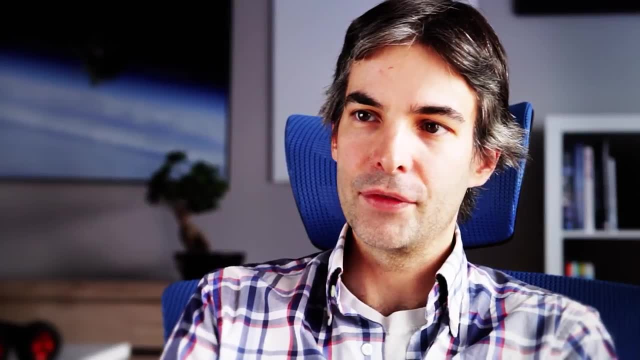 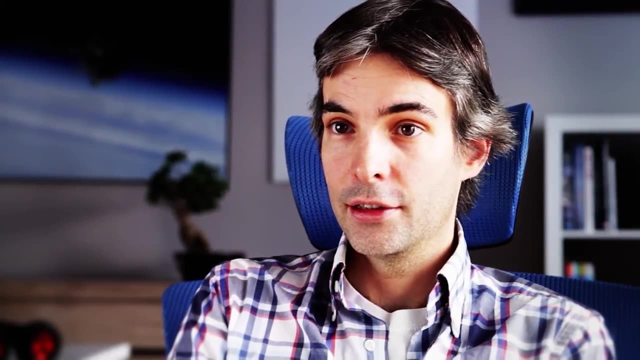 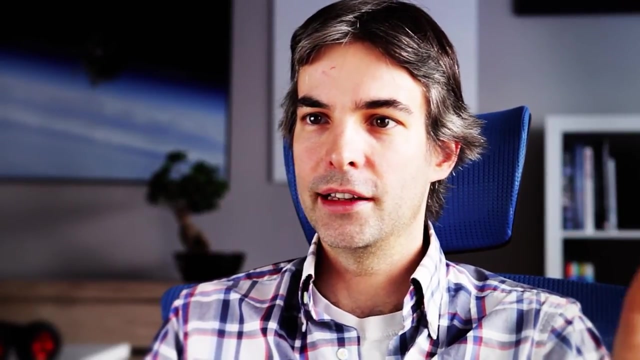 And that was a key thing here in proving the stability of our adaptive attitude controller. Because we needed to have a dynamics model with three inputs and three outputs only. So our three inputs in that case were the three control input torques. So one torque about the x-axis, one torque about the y-axis, and another torque about the z-axis as calculated by the attitude controller. 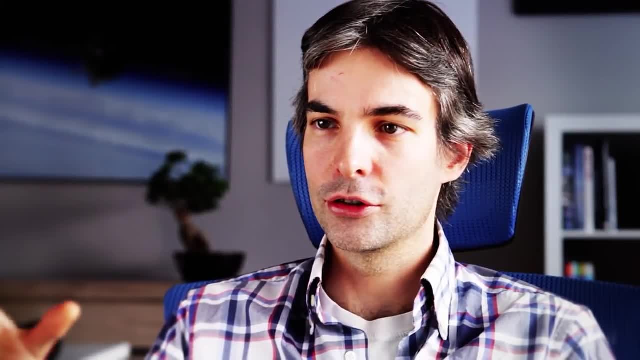 Whereas the output of the system we're controlling, in that case a spacecraft, were a three parameter vector 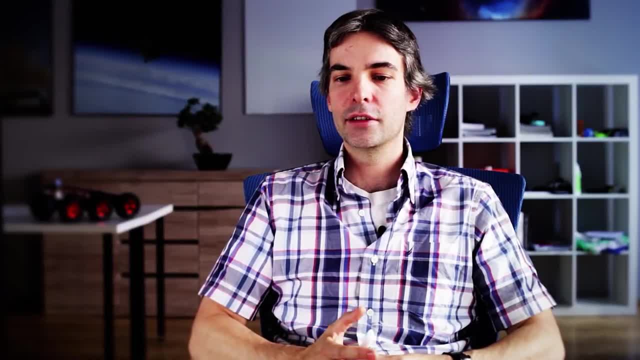 thanks to the MRP kinematics representation. 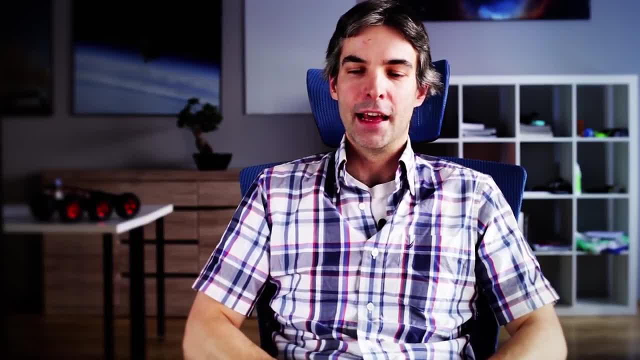 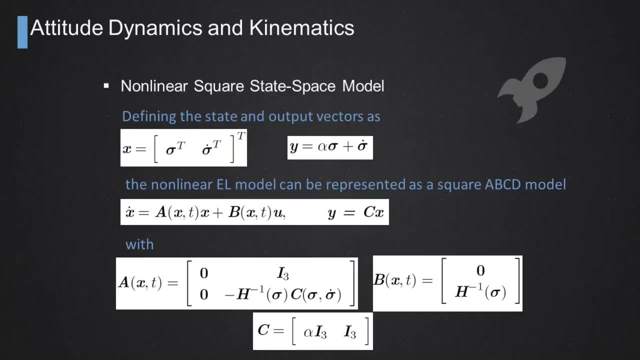 So three inputs, three outputs. And then what we did to ease up the development process was to reformulate the whole dynamics kinematics into a neuro-Lagrange dynamics model, non-linear dynamics model, which is widely used in robotics. 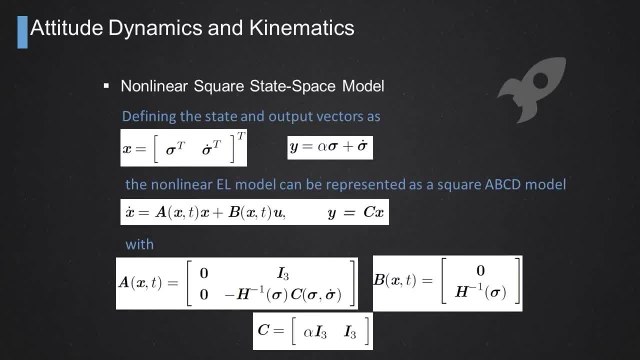 So you have your inertial matrix H, which is function of the current attitude, as represented by the MRP parameters. 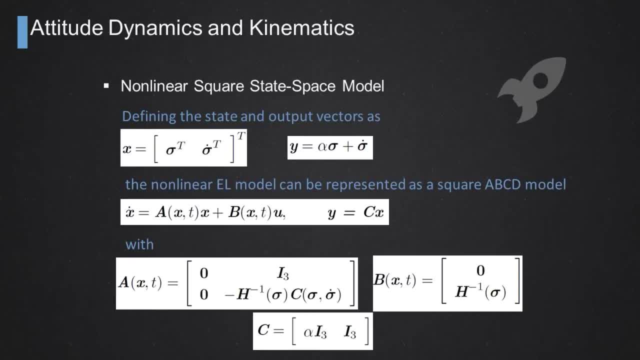 And you have your Coriolis matrix, which is function of the current attitude and the rate of change of the attitude. 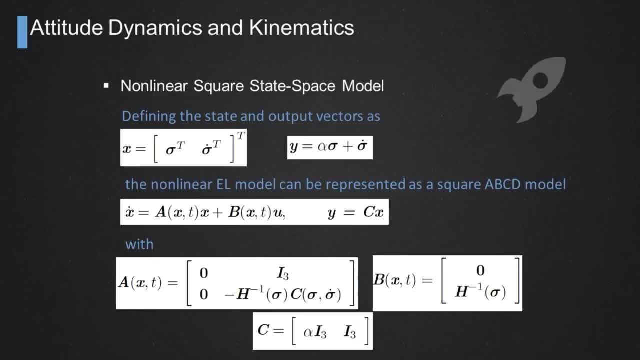 That's sigma and sigma dot. Next, we had to define the dynamics model as a square system with three inputs, three outputs only. 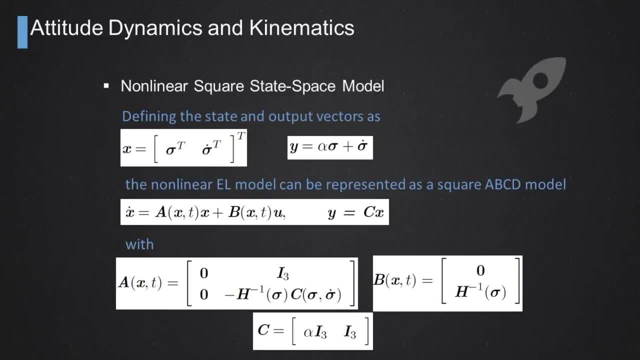 And we did this by combining the attitude and the rate of change in the attitude together into a single signal, such that we could model the output of our system with three components only. So this way we don't really need to know independently the attitude and the rate of change of the attitude. All we need to know is the summation of the two together. 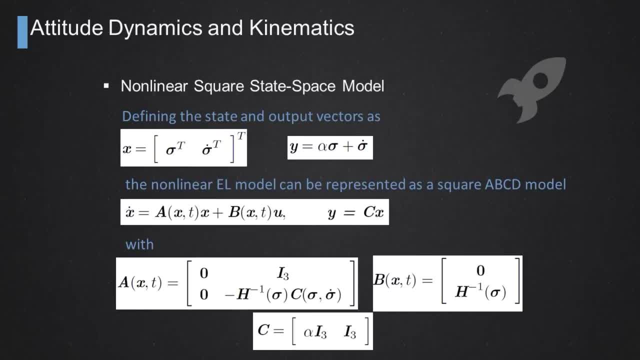 Again, we reformulated the whole thing as a neuro-Lagrange model, as a square ABCD state space system. 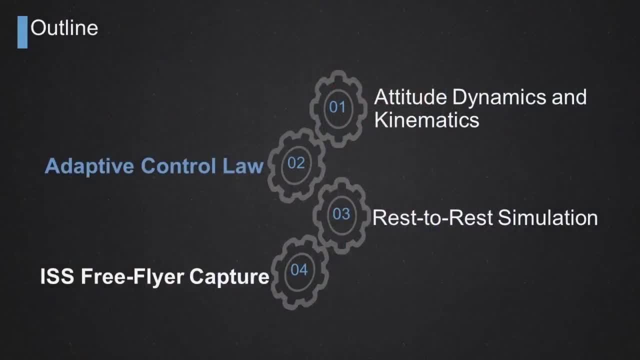 Alright, so now let's have a look at the actual adaptive controller that we developed. 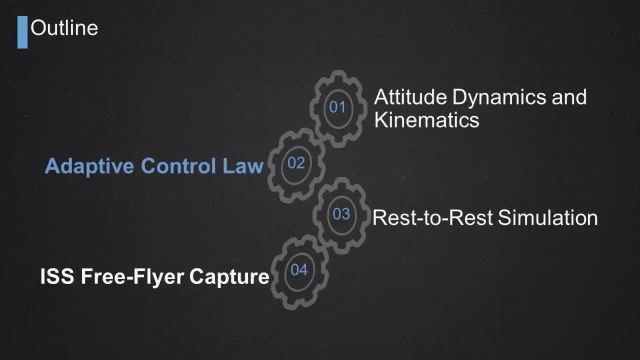 So that's the main innovation that we did in this work. 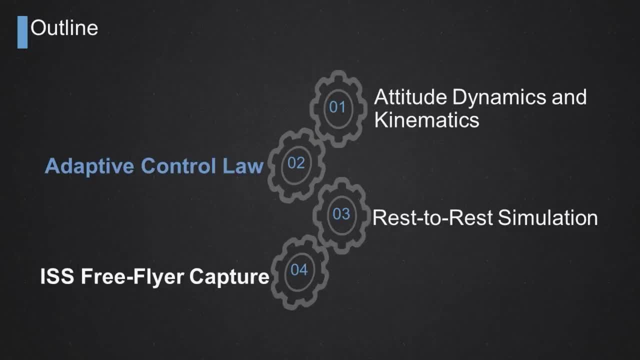 So here the control objective is similar to any other attitude control objective. 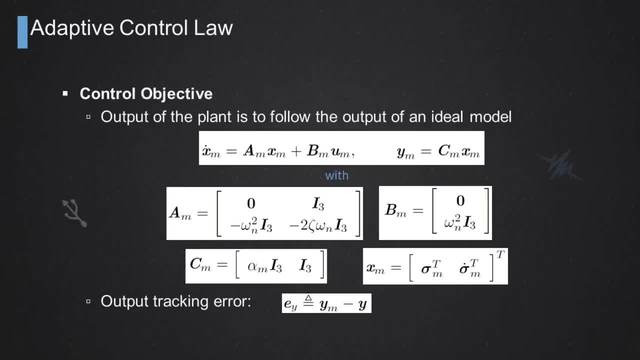 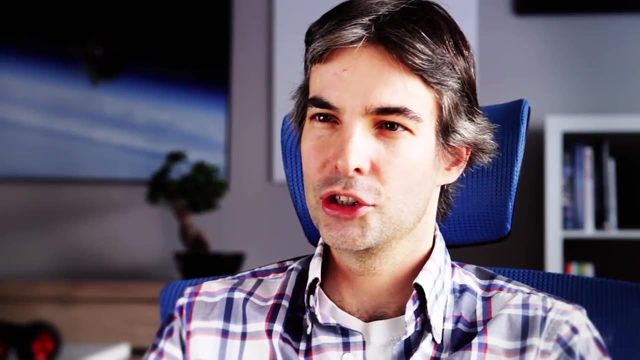 And that is that we wanted to have the output of the actual spacecraft in terms of attitude to follow as closely the output of an ideal model. The ideal model is equivalent to what I talked earlier in the other lecture, and that was a trajectory generator that was specifying the desired attitude profile as a function of time. 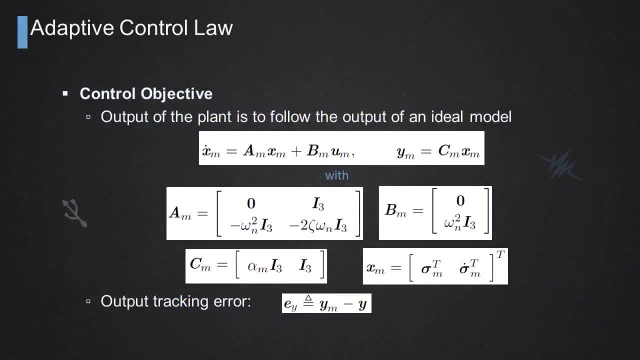 And this trajectory generator here was simply modeled as a second order differential equation that was 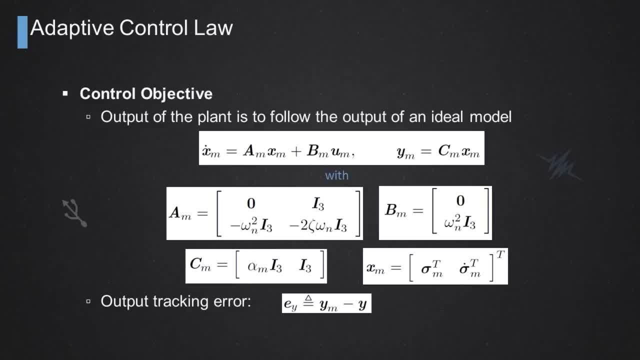 specifically designed to obtain a desired natural frequency of the closed-loop system as well as a desired damping ratio. And then to quantify this control objective we defined the output tracking error between this desired attitude profile noted as y subscript m and the output of the actual spacecraft. 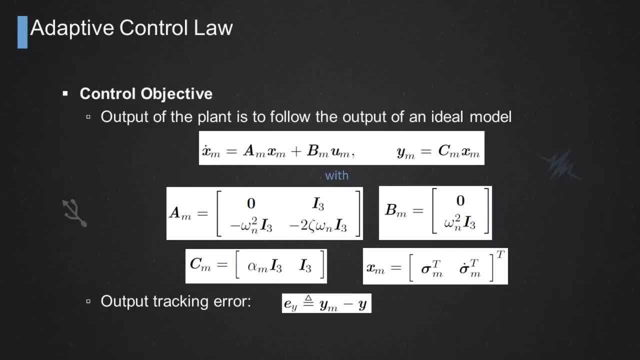 If you remember, that was a combination of the attitude and the rate of change of the attitude summed up together. So the difference between those two signals was our tracking error that our controller will aim at minimizing, again regardless of any uncertainties in the mass properties of the vehicle and also regardless of any external perturbations in that specific situation coming from the misalignment between the latching and effector 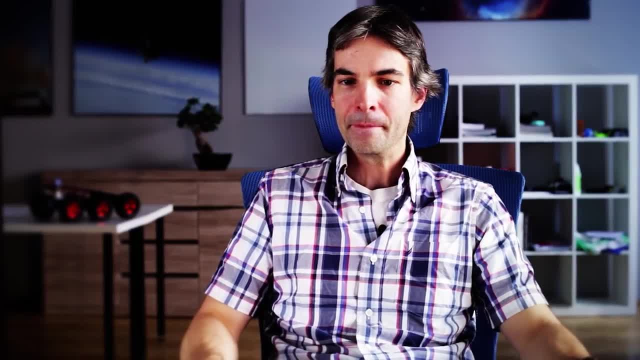 of the robotic arm and the grapple fixture on the target vehicle. 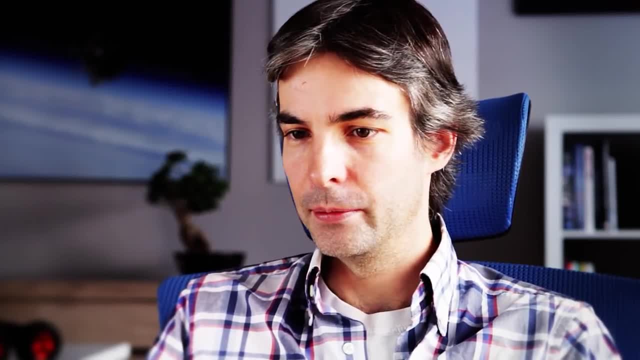 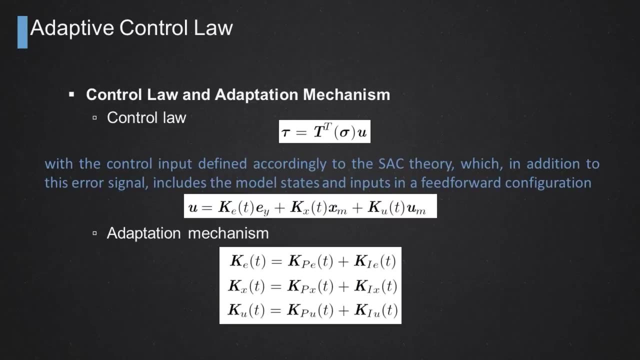 So we proposed a very simple control law for ease of implementation purposes. And we defined the control input torque so that's tau, again that's the output of the controller, that's the required torque to make sure that the attitude motion matches as closely as possible the desired attitude motion as simply being the kinematic matrix T that I briefly shown in previous few slides and U, which is a signal that was defined according to an existing adaptive control theory 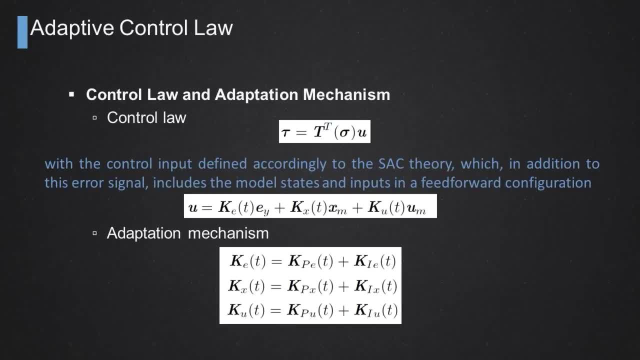 referred to as a simple adaptive control theory. And you see here the actual equation for U. So essentially U is calculated as a function of the tracking error EY so the greater the error and the greater the U signal will be as a result the greater the torque will have to be. 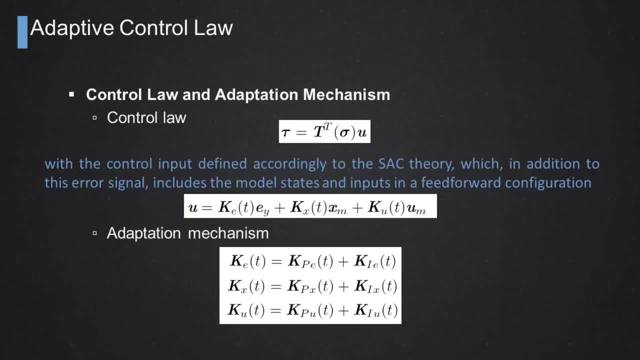 Not only its function of the tracking error EY but it's also function of the desired state vector of the ideal model and also function of the user inputs or if you will the input vector of this ideal model. So these are the signals X subscript M and Y subscript M as well. 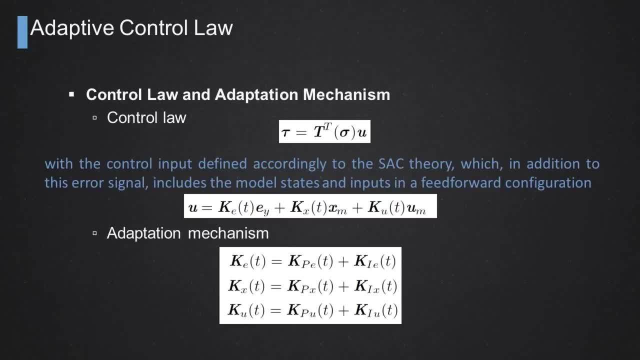 And the key thing here is that unlike traditional controllers that use fixed gain control matrices, here we decided to use time varying control gain matrices. That is the E, Kx and Ku control gains. 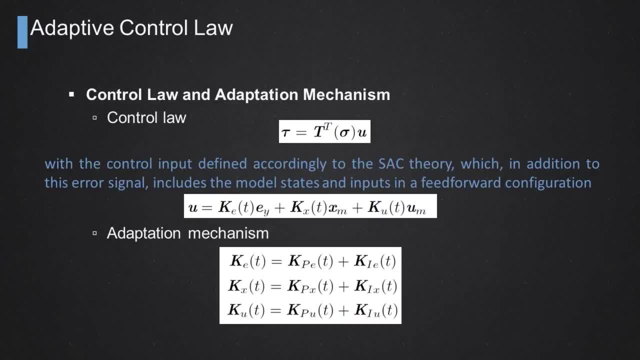 And by doing so that allows the controller to modify its behavior in real time according to the current tracking situation. And the adaptation mechanism for each of these three gains was broken down into a proportional term plus an integral term. 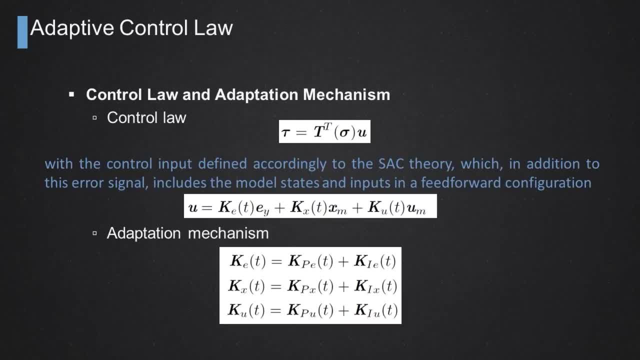 So these are a Kp and a Ki components as shown in the three bottom equations here. 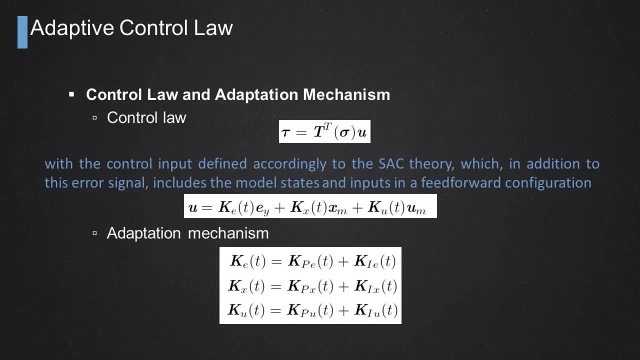 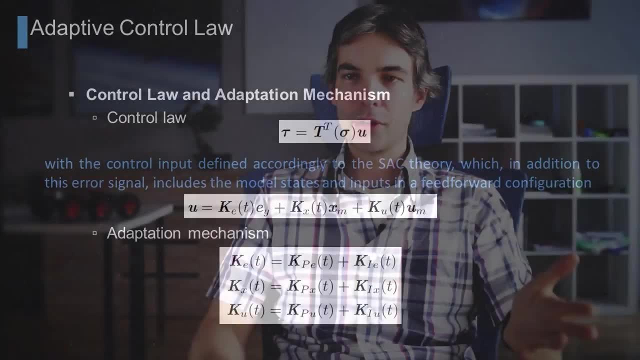 So all these proportional and integral components are adapted as follows here. I won't go into the details but again the key point is that they are all function of the output tracking error between the desired attitude and the current attitude. 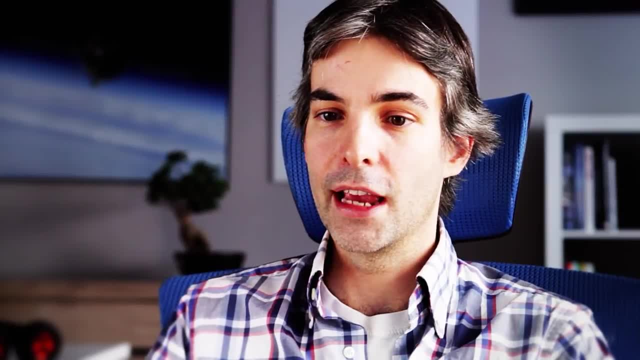 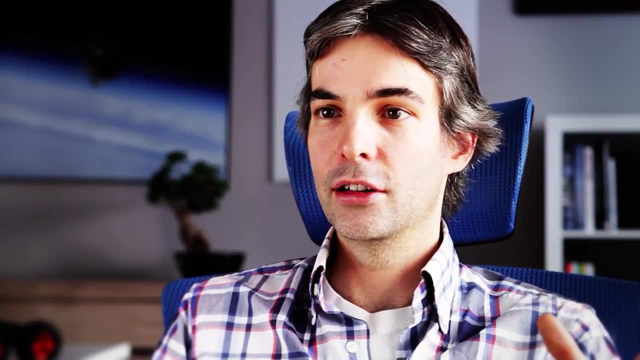 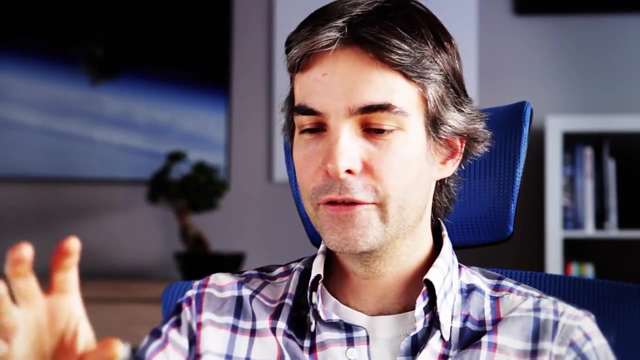 So the greater the output tracking error is, the greater the gains will have to be and in turn the greater the use signal will be and finally the greater the control input torque will have to be. So the greater the error, the more torque you need to apply onto the side light to make sure that it follows the prescribed or the desired trajectory. 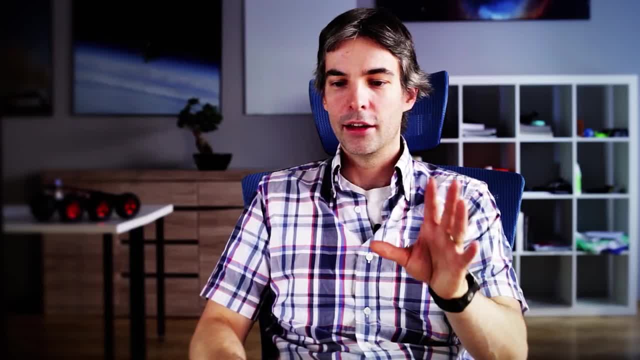 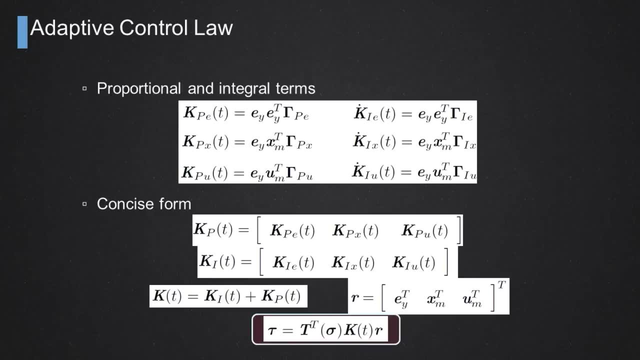 And the whole controller can be written concisely as shown here in the red box with K function of time being the total adaptive control gain as defined in the equations here. 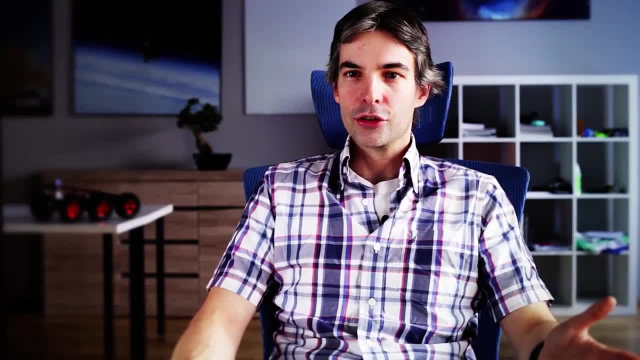 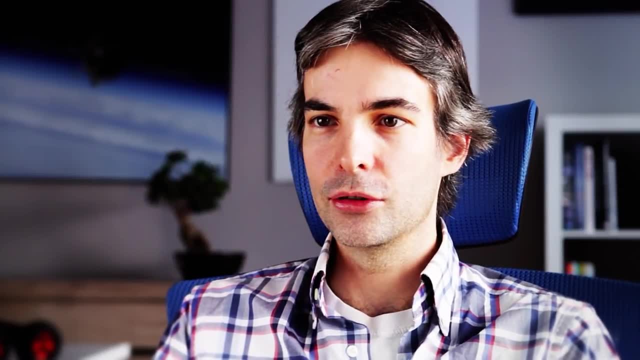 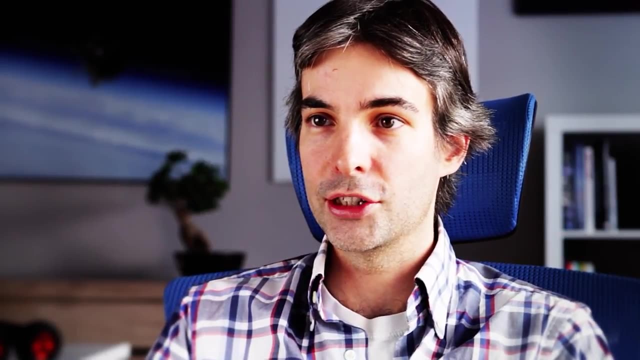 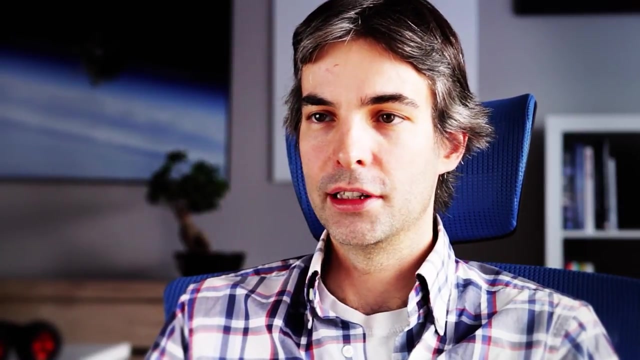 So whenever you're dealing with adaptive control techniques you do need to ensure that the closed loop control system is stable. Now because the adaptive control gains are free to various functions of time, of course you don't want them to become unstable, otherwise the whole spacecraft will start oscillating in an uncontrolled way and might eventually diverge completely resulting in a mission lost eventually. 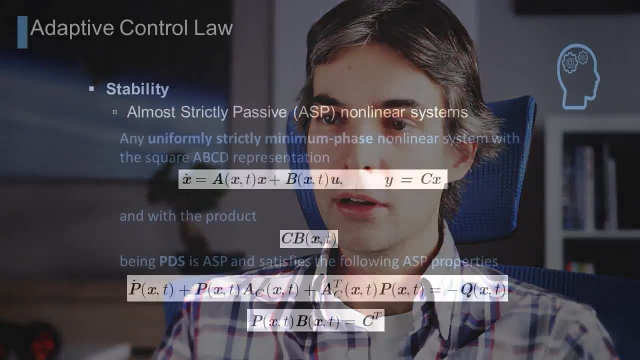 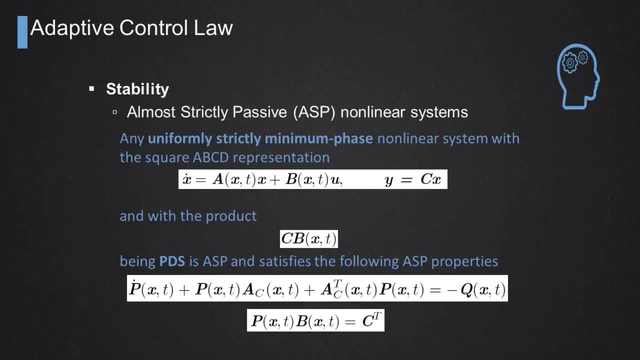 So one key aspect in ensuring that our adaptive controller was stable in closed loop was to first ensure that the closed loop system was almost strictly passive. So that's a property of non-linear systems that says that if your system is strictly minimum phase so that's another way of saying that all the zeros are in the left hand side plane, the complex plane if you're familiar with linear 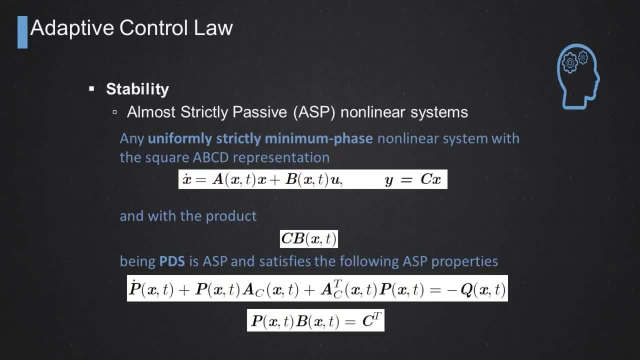 control theory. So that's one of the criteria that you have to check to make sure that your closed loop system is almost strictly passive. And the other one is that the product of the output matrix C with the input matrix B is positive definite symmetric.